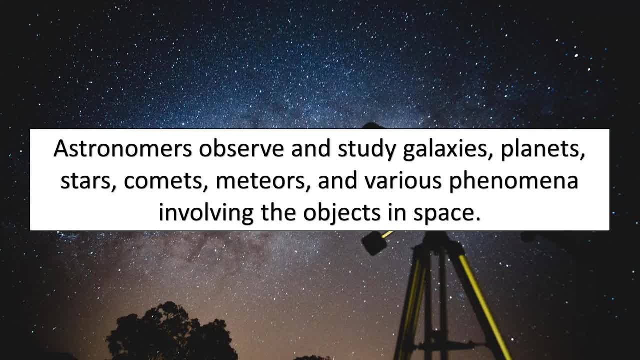 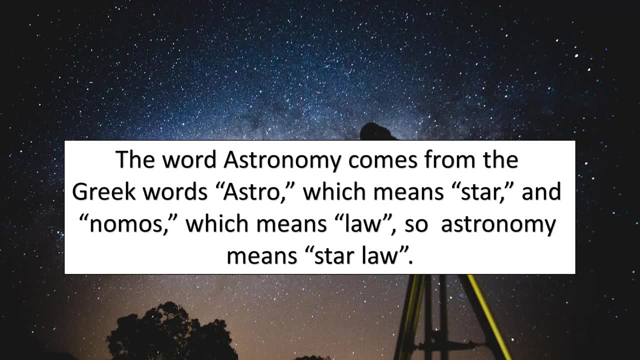 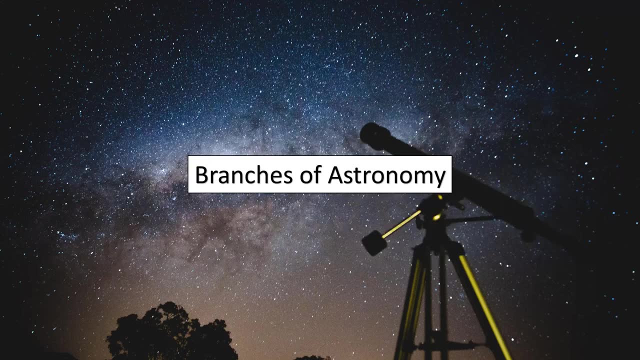 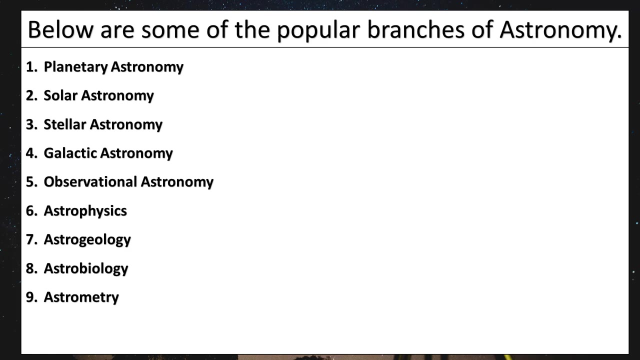 meteors and various phenomena involving the objects in space. The word astronomy comes from the Greek words astro, which means star, and nomos, which means la. So astronomy means star, la. Now we are going to see different branches of astronomy. Below are some of the popular branches of astronomy: Planetary Astronomy, Solar Astronomy. 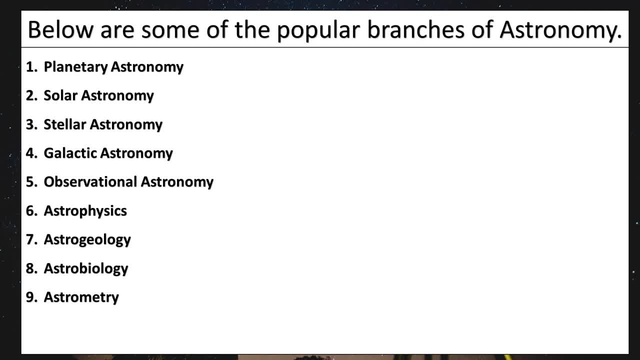 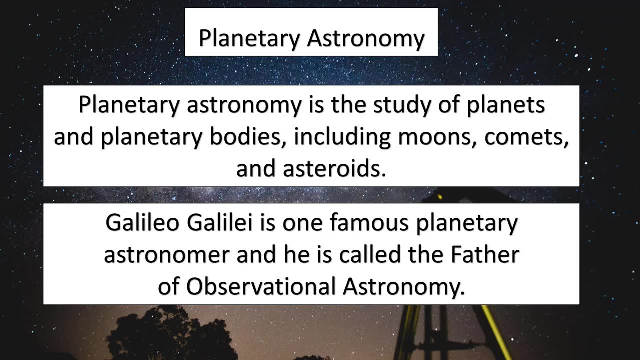 Stellar Astronomy, Galactic Astronomy, Observational Astronomy, Astrophysics, Astrogeology, Astrobiology and Astrometry. Let us see one by one in detail. Coming to Planetary Astronomy, Planetary Astronomy is the study of planets and planetary bodies, including moons, comets and asteroids. Galileo. 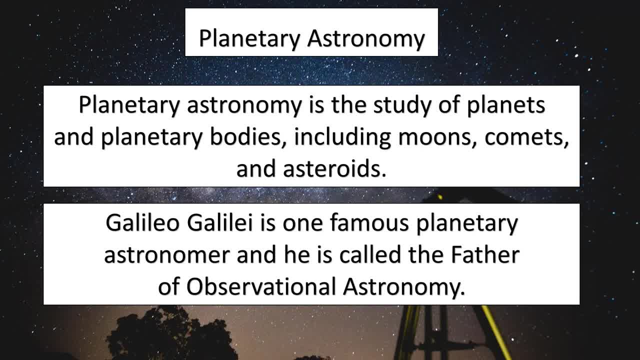 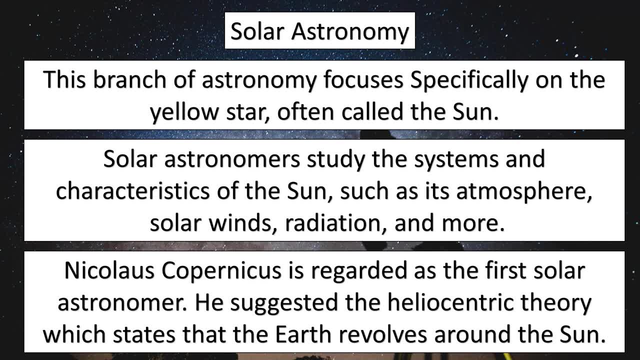 Galilei is one famous planetary astronomer, and he is called the father of observational astronomy. Now coming to Solar Astronomy, This branch of astronomy focuses on the yellow star, often called the sun. The collection of every planet organization based on sun has a scientific background. 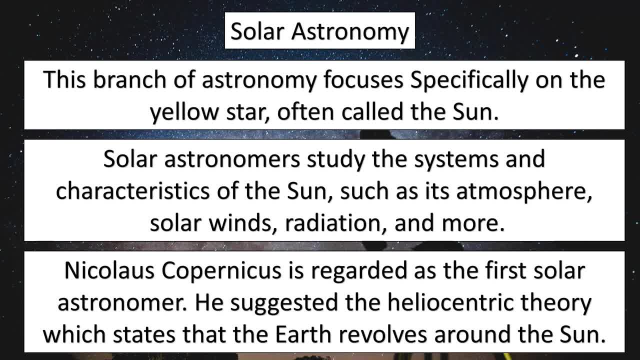 Thisiao Shoutout️. screening does not allow viewers to study and read recordedfonets of partner planets. On restoration of very important planets, there are several research instruments, such as empathy systems, whereas regarding observational astronomy, the databases are a bit more complicated. It has been observed that that they use breathing things. 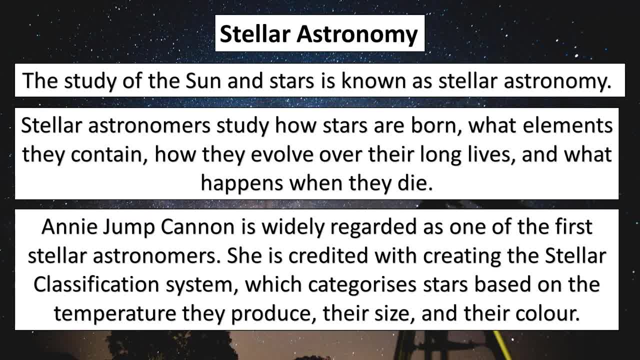 Now coming to stellar astronomy. The study of the sun and stars is known as stellar squid Stellar Astronomy. Stellar astronomers study how stars are born, what elements they contain, how they evolve over long lives and what happens when they die. Annie Jump Cannon is widely regarded as one of the first stellar astronomers. 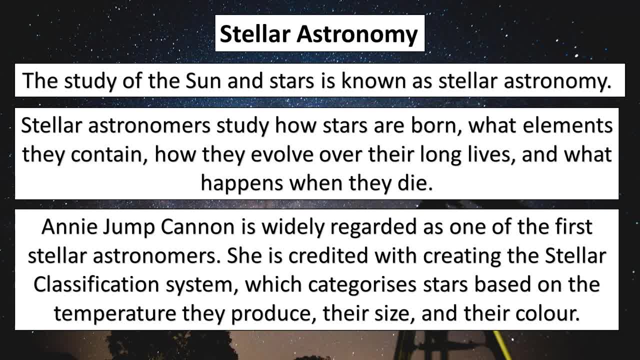 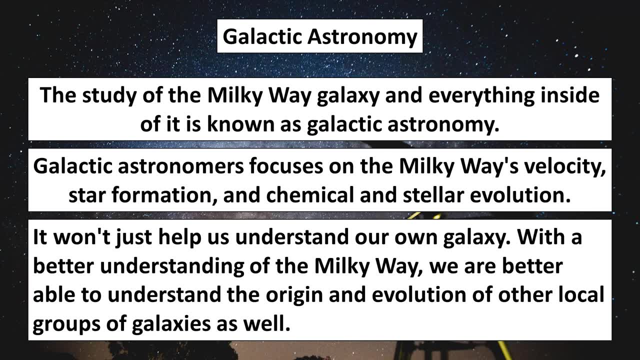 She is credited with creating the Stellar Classification System, which categorizes stars based on the temperature they produce, their size and their color. Galactic Astronomy: The study of the Milky Way, Galaxy and everything inside of it is known as Galactic Astronomy. Galactic astronomers focuses on the Milky Way's velocity, its orbit and its orbit. 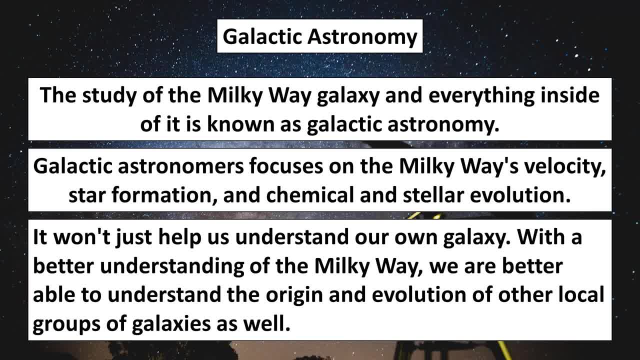 It is the source for gravity, stars and other elements. It will not only help us to understand our own galaxy, but if we understand the Milky Way better, we can better understand the origin and evolution of other local groups of galaxies as well. 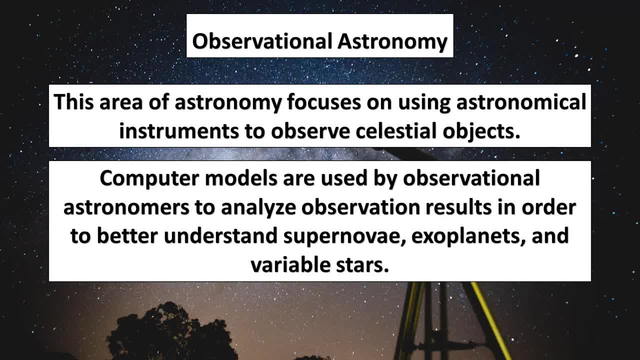 Now we are going to see Observational Astronomy. This area of Astronomy focuses on using astronomy and its organization to measure distances around the galaxy. astronomical instruments to observe celestial objects- Computer models- are used by observational astronomers to analyze observation results in order to better understand supernovae, exoplanets and variable stars. 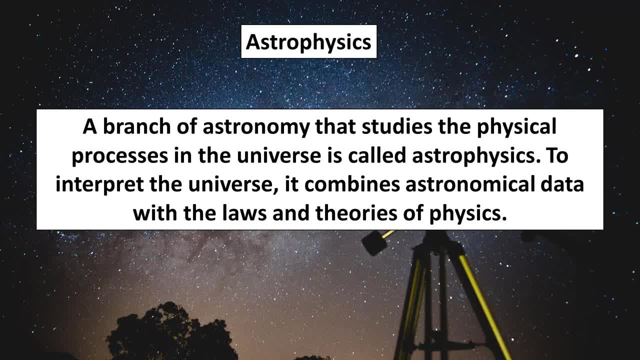 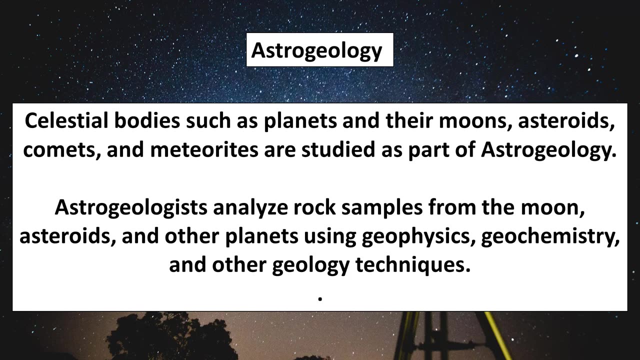 Now coming to Astrophysics. a branch of astronomy that studies the physical processes in the universe is called Astrophysics. To interpret the universe, it combines astronomical data with the laws and theories of physics, Astrogeology, Celestial bodies such as planets and their 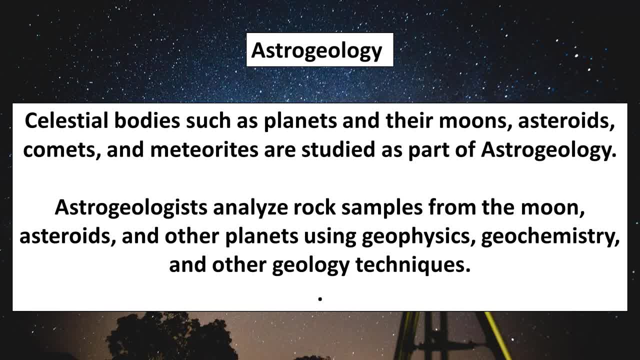 moons, asteroids, comets and meteorites are studied as a part of astrogeology. Astrogeologists analyze rock samples from the Moon, asteroids and meteorites. Astrogeologists analyze rock samples from the Moon, asteroids and meteorites. 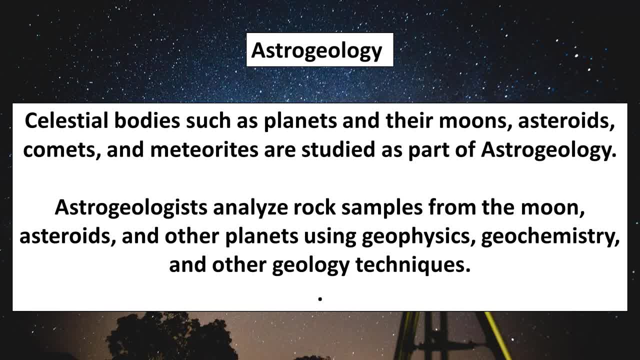 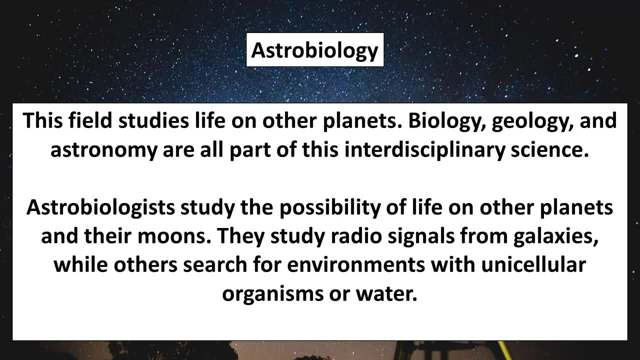 Asteroids and other planets using geophysics, geochemistry and other geology techniques. What is Astrobiology? This field studies life on other planets. Biology, geology and astronomy are all part of this interdisciplinary science. Astrobiologists study the possibility of life on other planets and their moons.